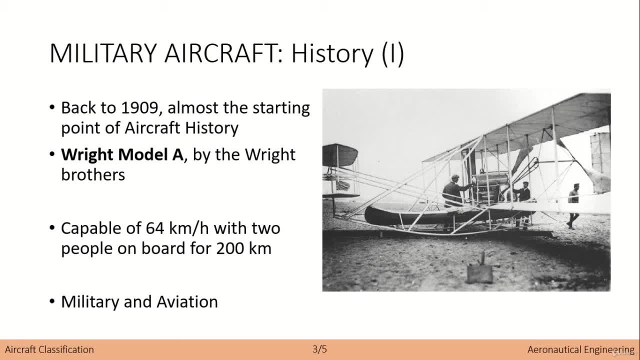 Okay, so quite an interesting first airplane, considering it was back in 1909. So basically the beginning. I think the first tests for The Wright brothers aircraft were in 1905 or something like that And as you can see as 1909, it was kind of operational. 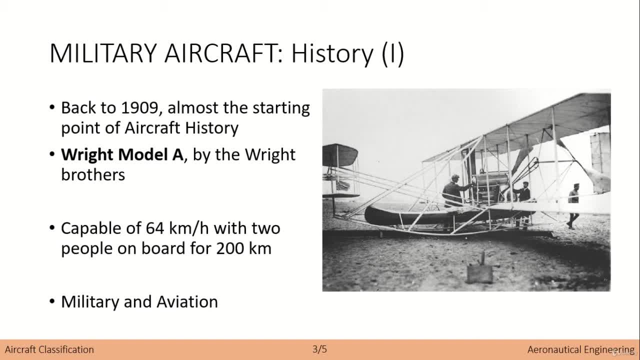 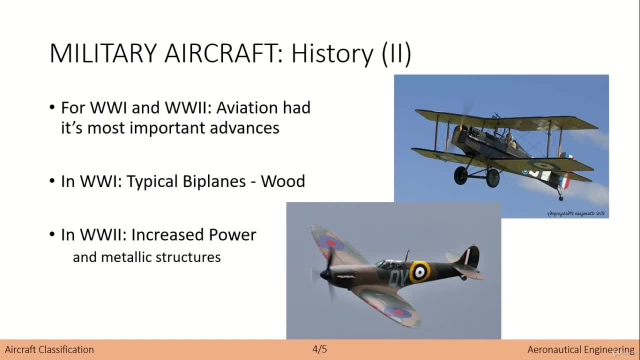 Okay, just with some modifications of course, but it was kind of a good start for military aircraft. Okay, as you can imagine, for World War I and World War II, aviation had a lot of important advances, Okay. Okay, Here you have the World War I typical biplanes. 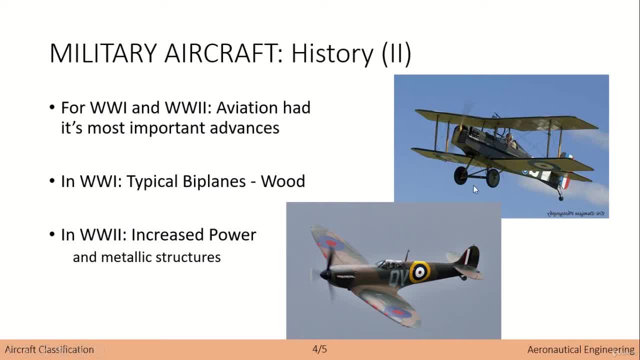 Okay, which were based especially on wood, were developed and were constructed based on wood because wood was kind of a lightweight material in the time. You can imagine that having a Boeing or an Airbus right now made of wood would probably not be the best idea. 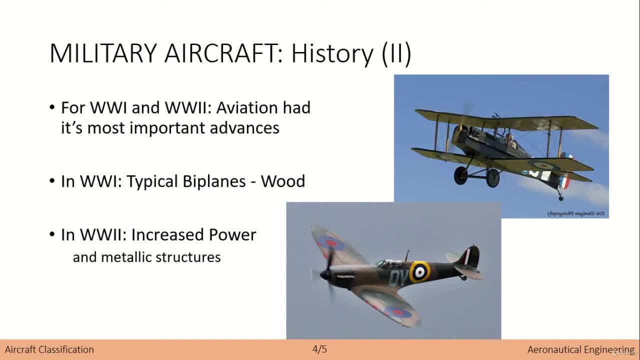 Okay, for the properties of the wood, of course, And, as you can see, the idea is that most It is typical in the World War I that actually planes had this kind of biplane configuration, as you can see, Which is kind of interesting because basically the idea was that the motors, the engines that they had, 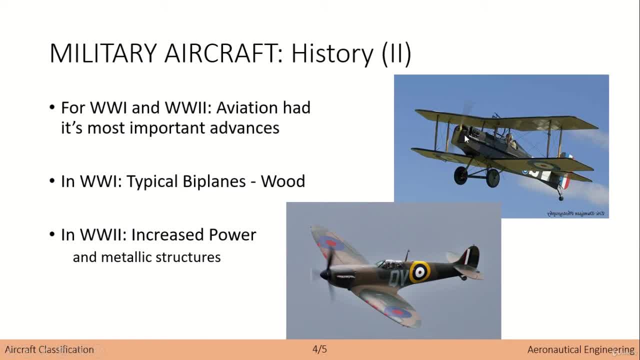 were not powerful enough to provide very high speeds And, as we will see in the aerodynamic part, it was essential to have very high speeds. Okay, So the idea is, if you have low speed, then you need to have very high speeds. 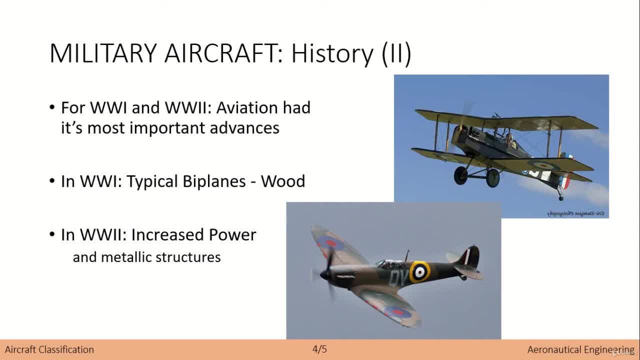 You need more surface, okay, So that you can provide a lift and therefore the aircraft can actually fly. So this was the idea, okay? For World War I, the engines were not powerful enough, so they needed more surface. What happened in World War II? 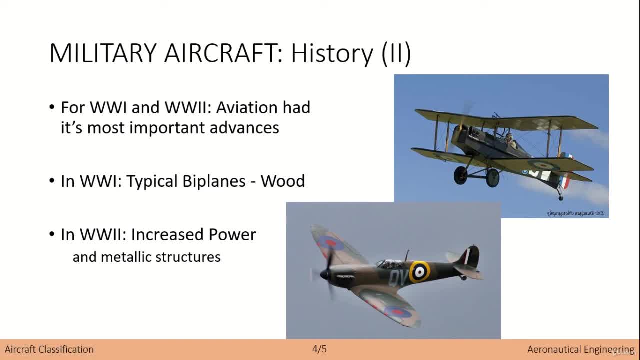 Well, the idea is that especially the metallic structures were introduced, And metallic structures- you may understand that- may be heavier, okay, than wood, But the structures were more solid. So in the end you needed more- sorry, less material, okay. 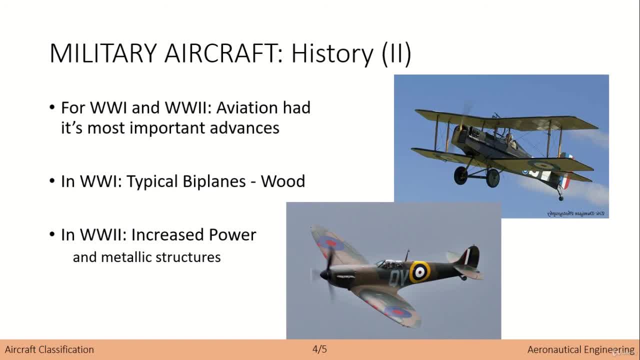 So less weight in the end. And of course, it had better properties. okay, It had more strength, it resisted more loads And therefore you could just develop one wing plane with a completely different configuration. This is kind of elliptic, okay. 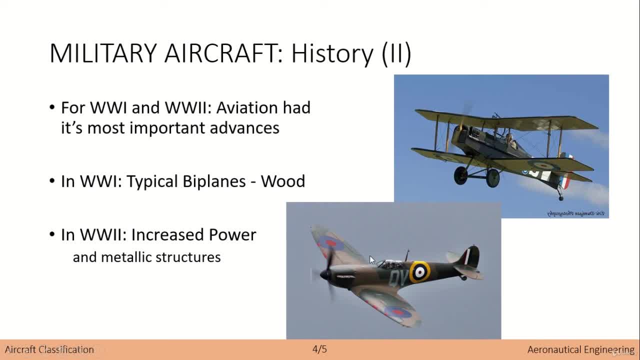 This is the elliptic of the Spitfire, which is very well known, And, as you can see, this is the Spitfire. And, as you can see, this is the Spitfire. This compares completely different to the first model. okay. 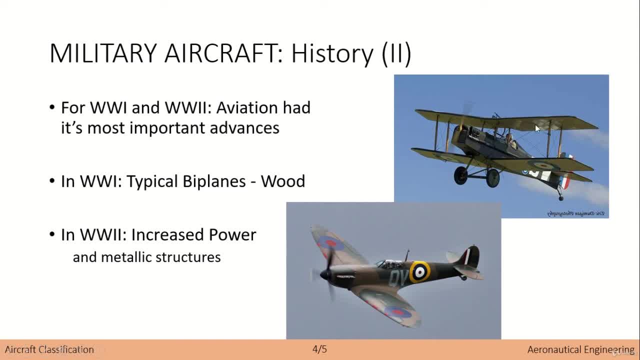 Of a typical biplane of the First World War. All right, As you can see. also, the motors, the engines that were used in World War II were far away, were just very, very much more powerful than the ones used for World War I. 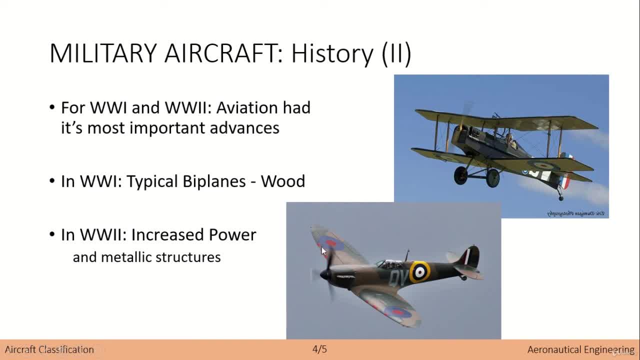 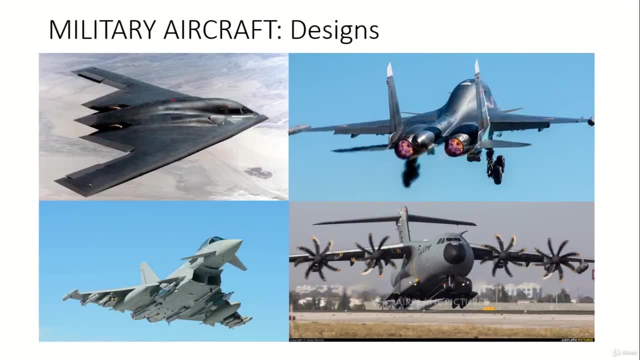 So this is why you have this kind of aircraft, which kind of resembles a more common aircraft that you would have right now. okay, so here you have several designs of military aircraft. it's quite interesting to note that the first one is a spy one. 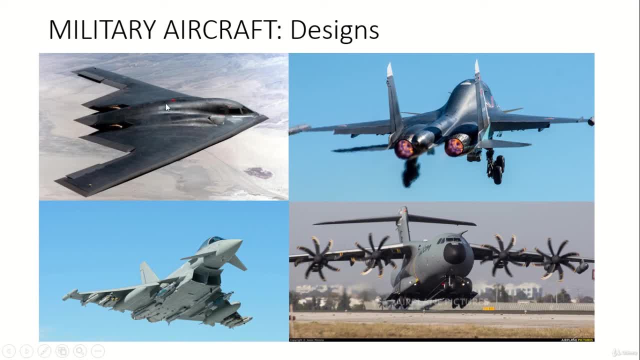 I think it's one from the United States. this kind of, of course, this kind of aircraft was something very experimental. you couldn't apply this to any other thing than just for spy or military operations. okay, it was a bomber also. here you have, I think this is a Su-35, it was one. 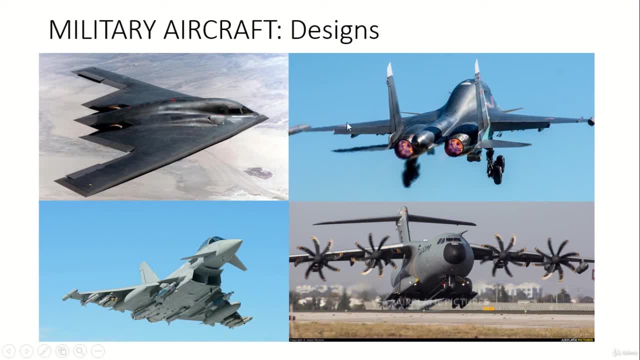 of the most iconic aircraft. regarding the Russian Air Force, okay, it is really, really capable. as you can imagine, the materials are very strong, they can resist very low, very much very high loads and therefore you have simply a very good aircraft. okay, you also have the typical Eurofighter. 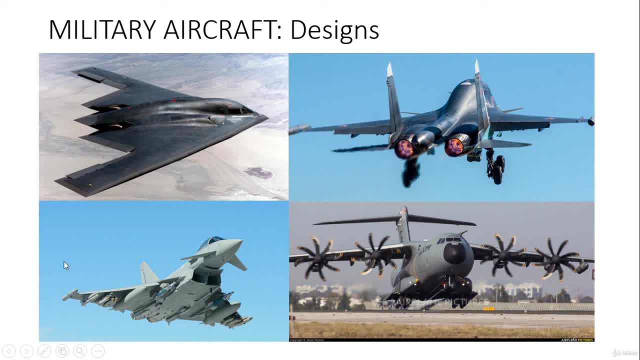 Typhoon Eurofighter, which is the one used for NATO, especially in Europe. okay, and here are some more aircraft. as you can see, this is a bit different. this is not a fighter, this is not an attack aircraft, but rather a bomber and kind of aircraft which can be used for transport means.